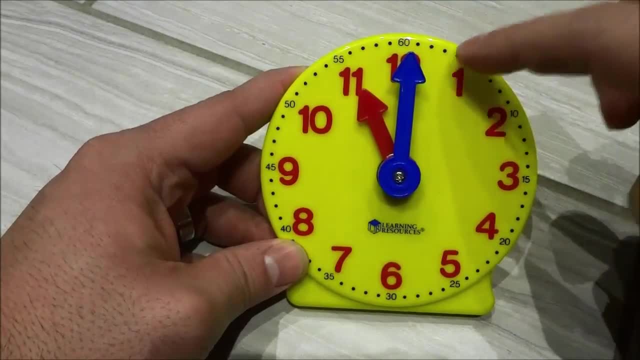 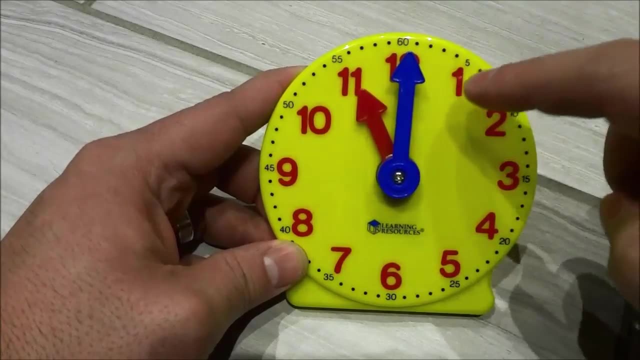 So this would be 5 minutes, this would be another 5 minutes, this would be another 5 minutes, and so forth. So in order to figure out how many minutes have passed at each big number, we need to skip count by fives. 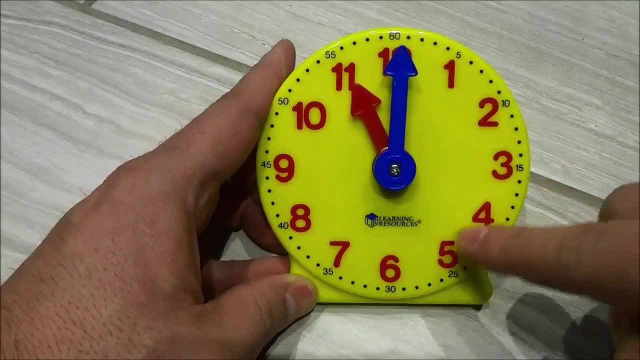 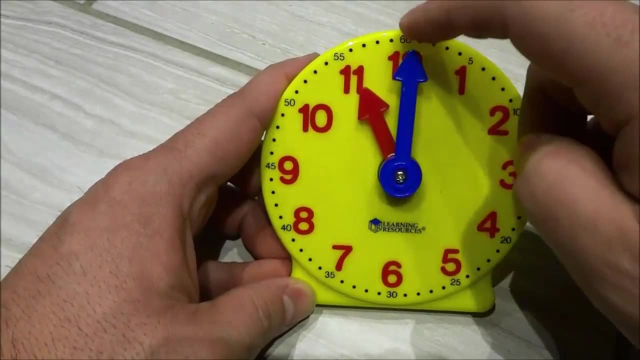 5,, 10,, 15,, 20,, 25,, 30,, 35,, 40,, 45,, 50,, 55, and then 60. But when we get to 60, it becomes o'clock. 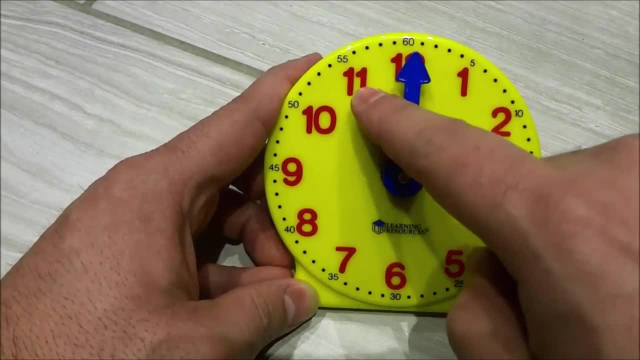 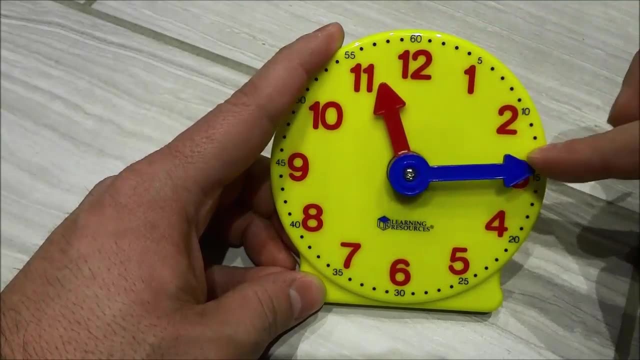 So this wouldn't be 1160, this would be 11 o'clock. So what I'm going to do is I'm going to move the minute hand to the 3 right here. okay, So we're gonna look at the small hand first and we're gonna look to see what hour it is. 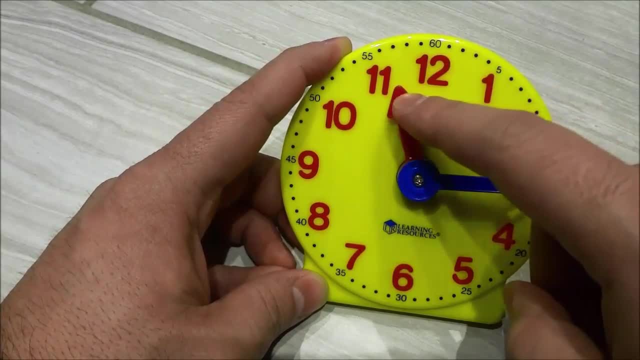 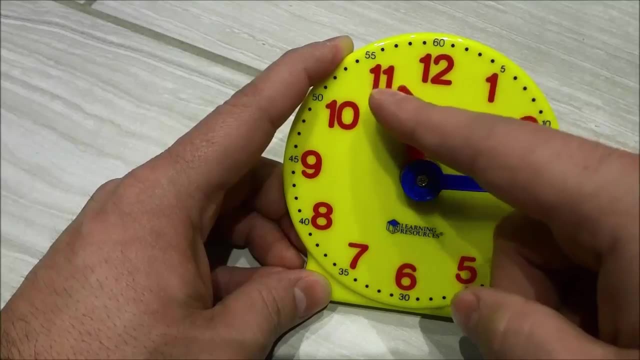 Now, it's not pointing at the 11, but it's also not pointing at the 12.. It is in between the 11 and the 12,. okay, So to figure out what hour it is, you're gonna see if it's pointed at a number. 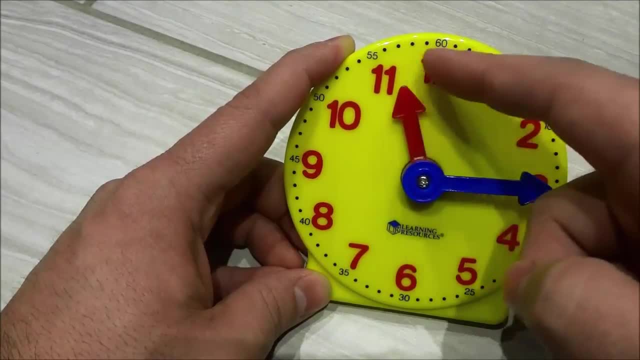 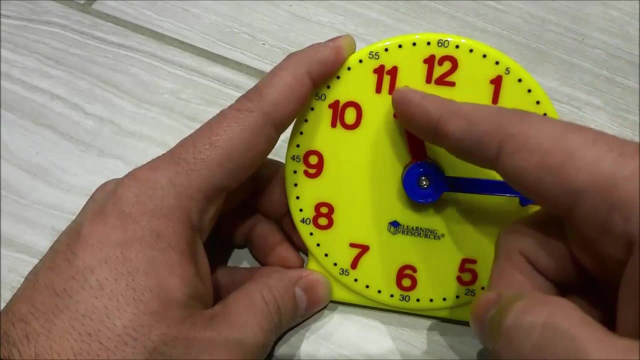 If it's not pointed at a number, you are going to go to the lowest next number. So right now, it's pointed right here. Sorry about that, That was just my oven telling me that it's ready. Right now, it's pointed right here. 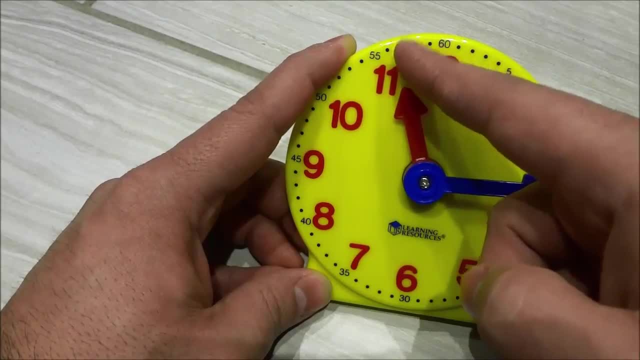 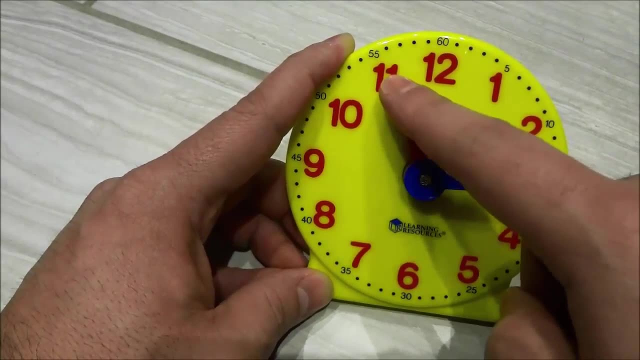 Right now, it's pointed right here. Right now it's pointed right here: You're gonna go to the lowest next number, So the next lowest number is 11.. Okay, just go to the next lowest number- 11- and then. so it's 11, and then we're gonna figure out how many minutes it. 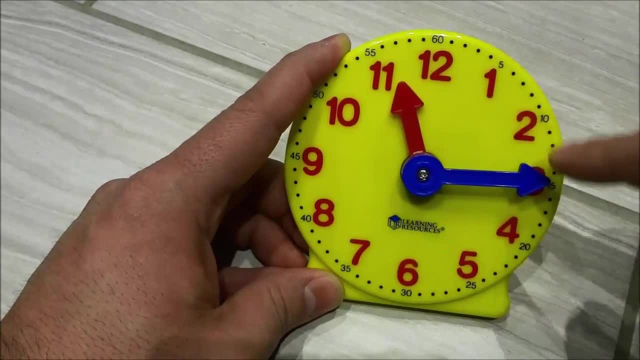 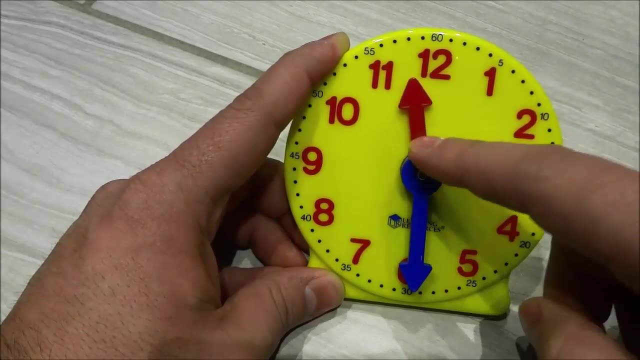 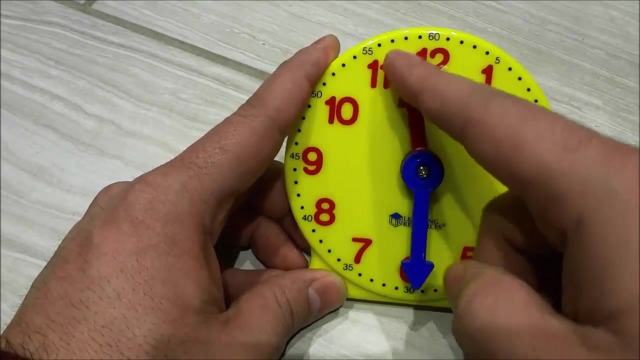 Is 11, then 5, 10, 15. it is 11- 15. I'm just gonna turn this a bit more. Okay, Now we're gonna look at the. we're gonna tell us figure out what time it is right now. Look at the small hand. We can see that it is pointed right here, which is in between the 11 and 12. 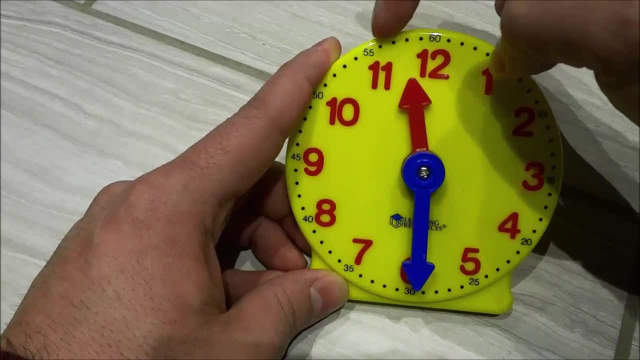 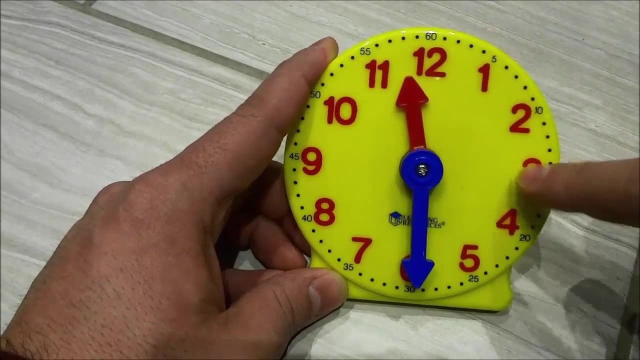 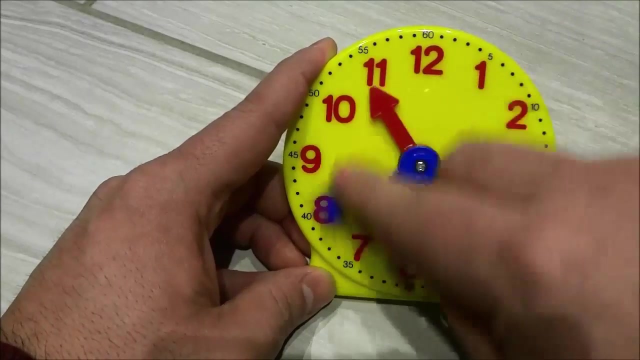 Okay, we need to go to the next lowest number, which is 11. It is 11, and then we're gonna figure out the minutes: 5, 10, 15, 20, 25, 30, It is 11, 30.. Okay, I'm just gonna spin this around just to move it once again. 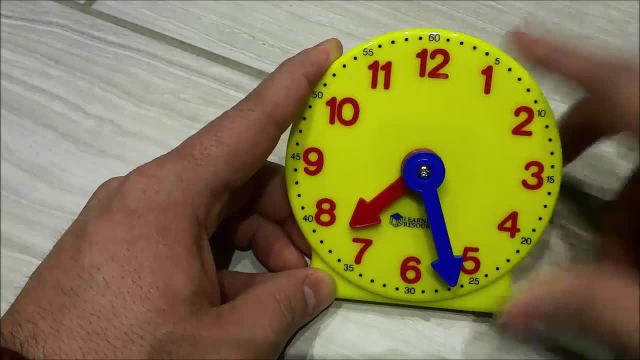 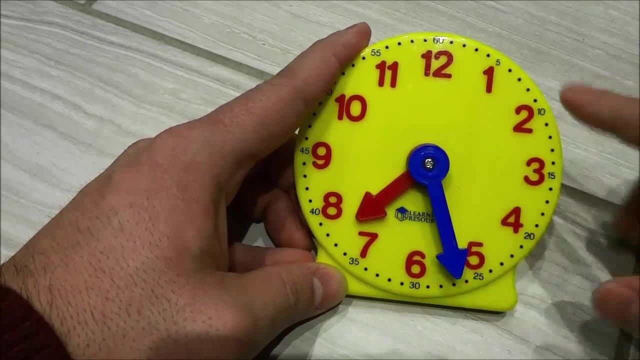 All right, so I'll bring it over here. Alright, now we're gonna do the same thing, but you can see that the minute hand, the big hand, is in between two numbers, So we can't stop when we skip count by fives. Let's start by taking a look at the hour hand right here. 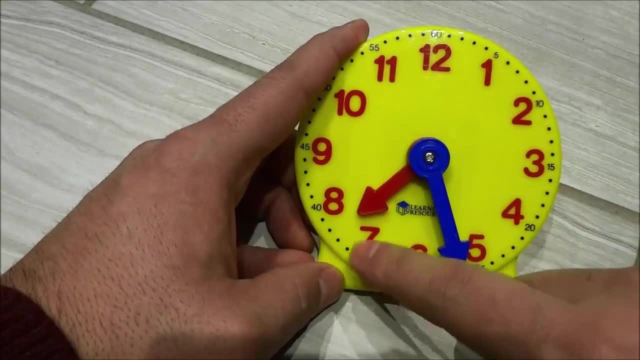 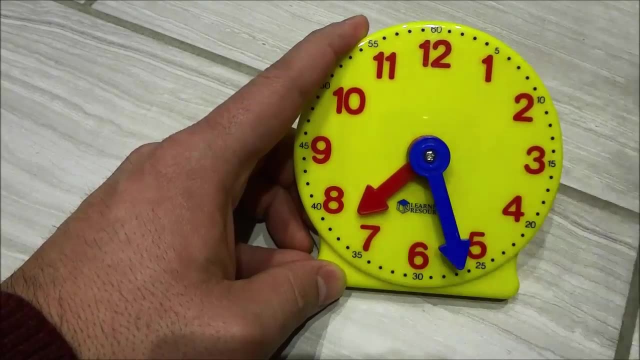 Okay, the small hand, the hour hand, is in between the seven and the eight, So the next lowest number is gonna be seven. So we know that the hour is seven and let's go ahead and count the minutes. 5, 10, 15, 20, 25. 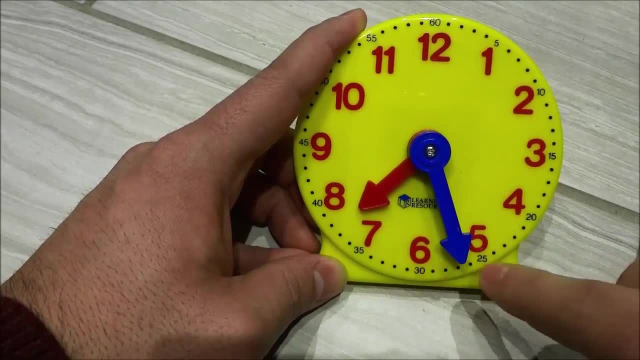 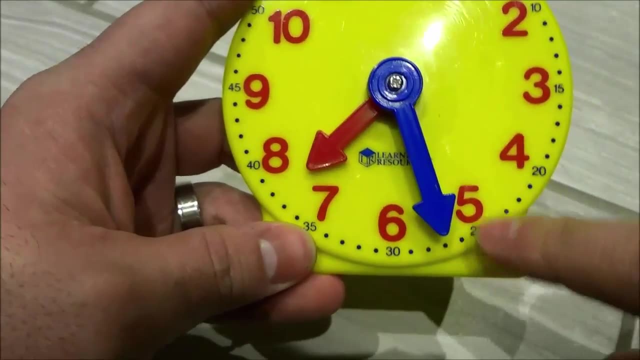 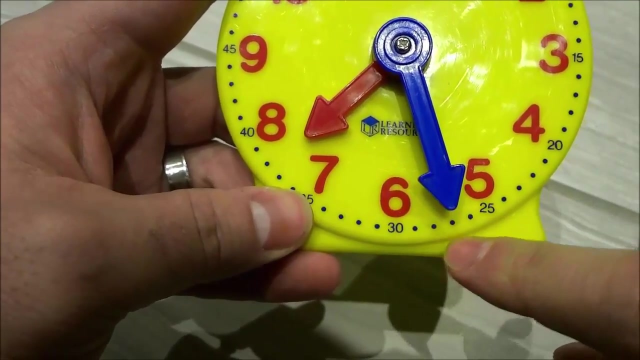 And 30 would be too much, 30 would be too far. So at 25, if you take a look at the minute hand, okay, you can see that it is past 25, but before 30. So we need to figure out how many small notches it has passed. 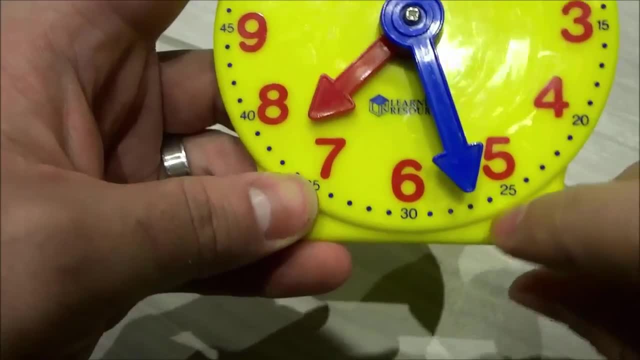 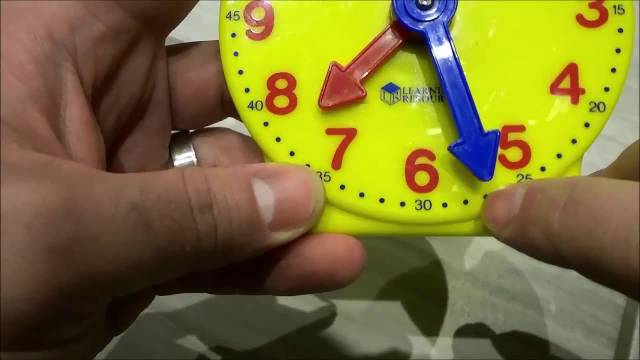 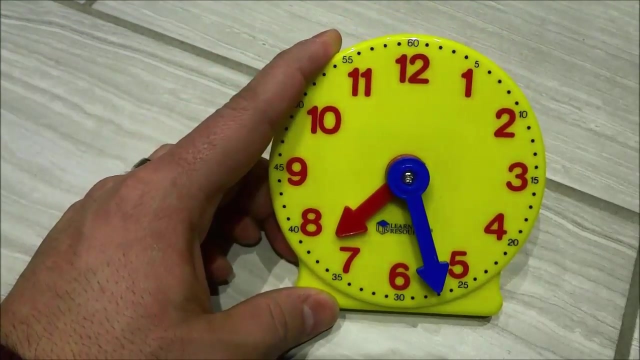 So 25, and each of these small notches counts as one: 25, 26, 27, once again 25, 26, 27, 27, the time is 7, 27 and that's basically it. in this video, I have shown you how to tell time and how to read a clock. 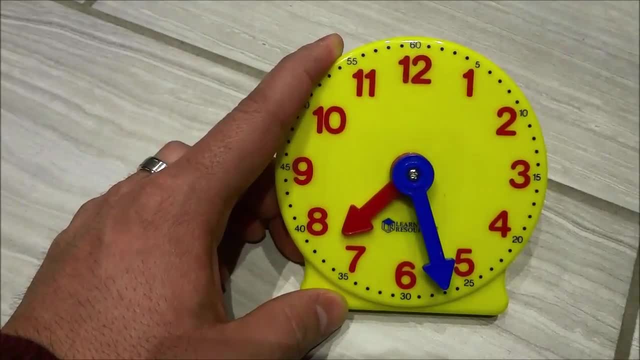 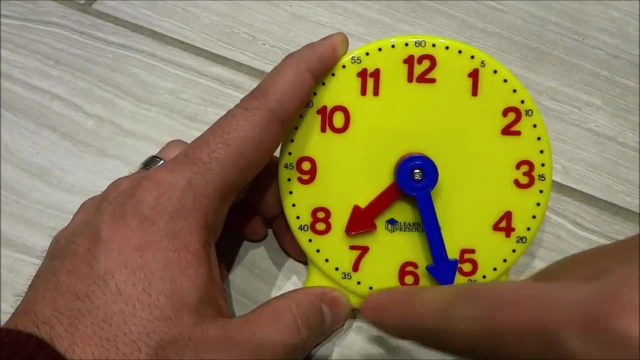 And just for the record, this is an analog clock, not a digital clock. So, basically, all that you have to do is figure out how. figure out how the clock works with regards to how it, the way That it goes around. know that this is the small hand, is the hour hand. 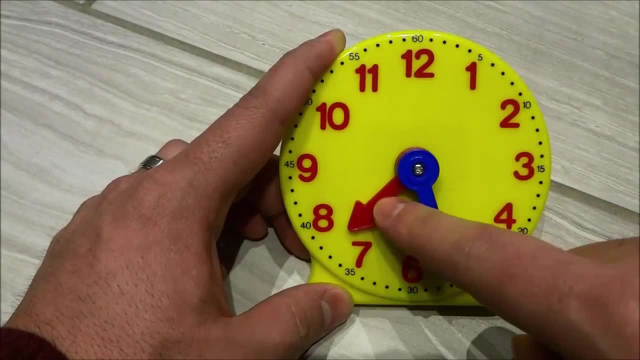 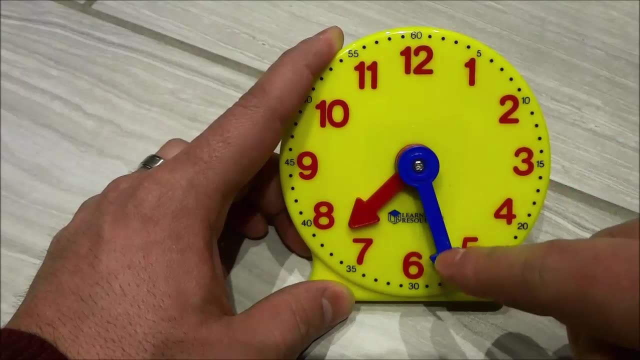 And the big hand is the minute hand, and then figure out what hour it is by looking at the small hand and where it is Pointing, and figure out what minute it is by looking at the the big hand and where it is pointing, and then just put them together. 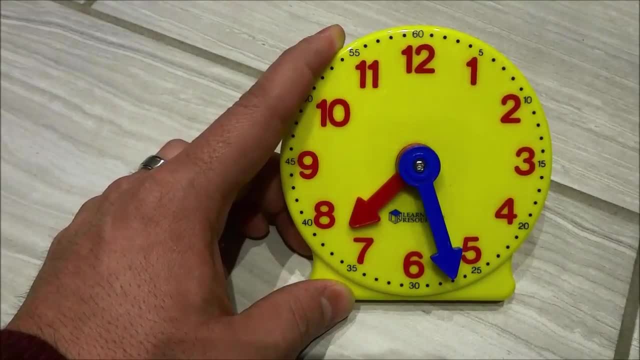 The small hand and the big hand where they are pointing. put the numbers together and that's all I have for you today. Thanks for watching.